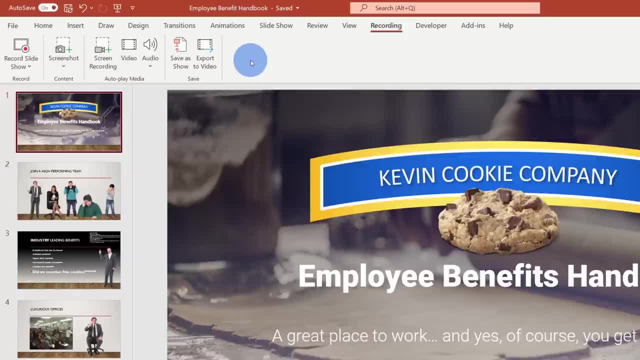 custom slide timings and maybe for the fun of it I'll even throw my video in so, as I'm explaining it, people can see me as I'm explaining it. On the Recording tab over on the left-hand side there's the option to record the slide show Here. if we click on the drop-down, you can start from the. 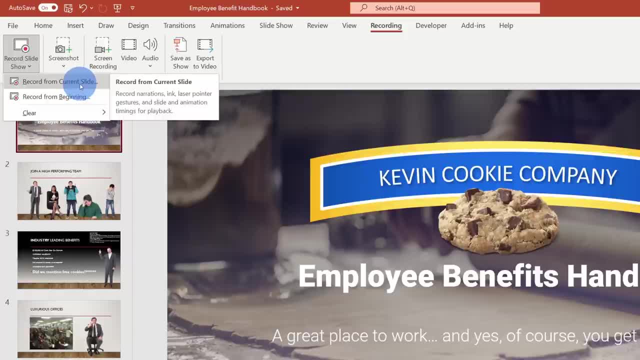 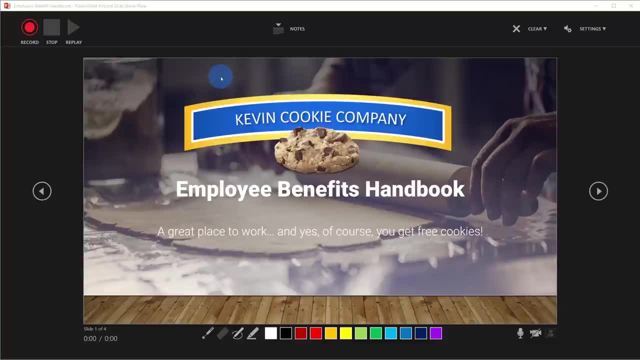 current slide or from the beginning. I'll just simply start from the current slide. It also happens to be the beginning. This drops us into the Recording tab. I'm going to click on this one to record the slide show interface, and there's a lot of functionality here, so I quickly want to. 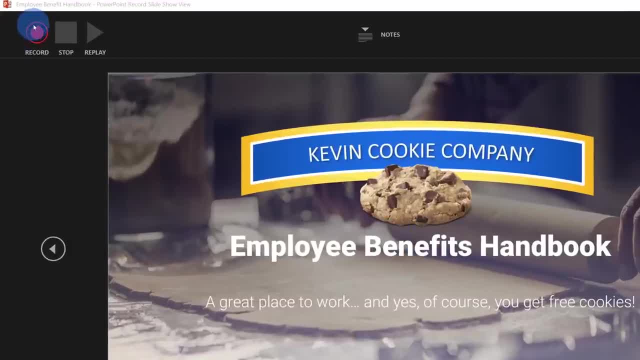 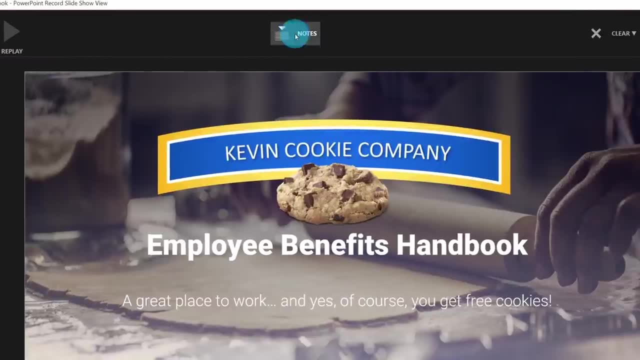 touch on what you can do with this screen. In the top left-hand corner you have this big record button and in a moment we'll use that to record narration on top of these slides. In the center you can expose your notes if you need a little bit of assistance as you're talking through it. 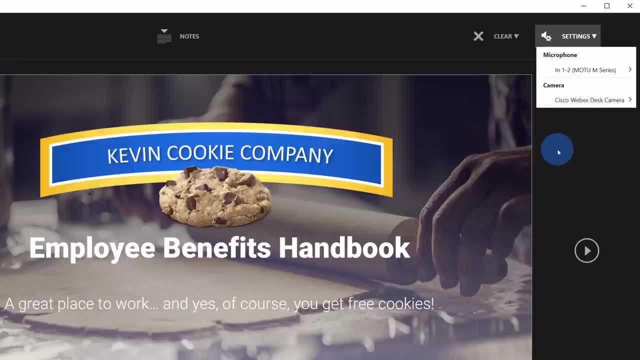 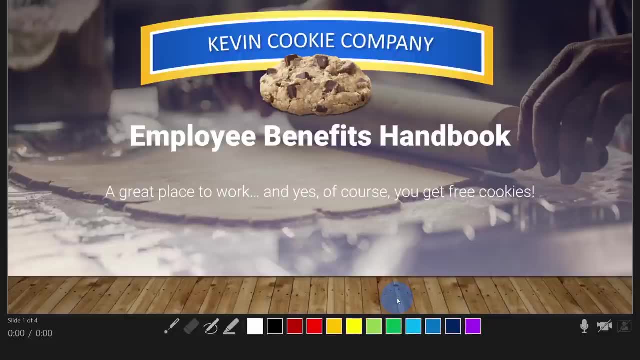 Over on the right-hand side. you can choose the microphone, You can choose the camera that you want to use, and then down below we have all of the standard PowerPoint annotation tools. As part of that, I include my video. Down here in the bottom right-hand corner, I can toggle my camera on. Hello. 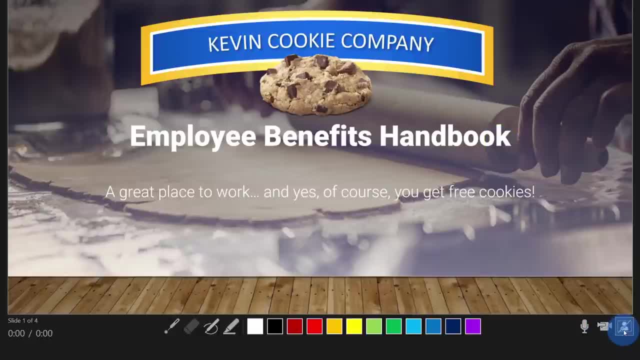 now you can see me. Look at that, And I could also hide my preview if I don't like seeing myself as I'm explaining things, or I could show myself, and I don't mind having my video down there. It's good to just orient myself to where that video is. And over here once again I have all of my different. 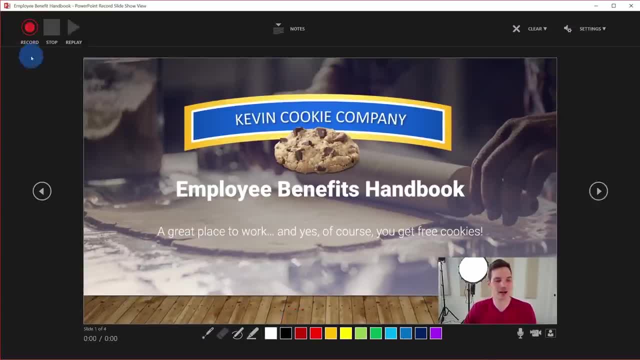 annotation tools. So I'm now ready to record. So I'll go to the top left-hand corner and I'll click on the record button Now. right now I see a countdown timer letting me know that the recording is active. So here I can select my tools and here I could go in and I could point at things on my 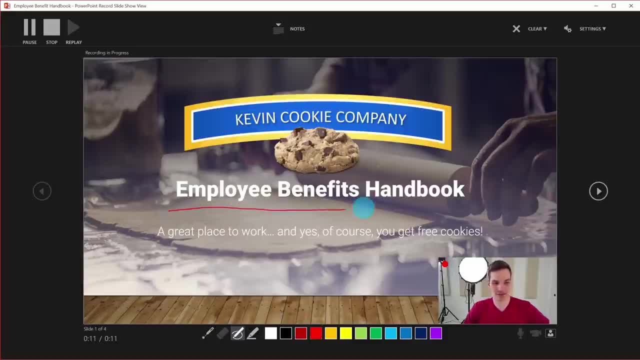 slide. I could also select the pen tool and I could annotate different things, So you could actually make this a very rich video with annotation, So it really makes it easy to explain things. Once I'm done explaining what's on this slide, I'll go over and click to advance. 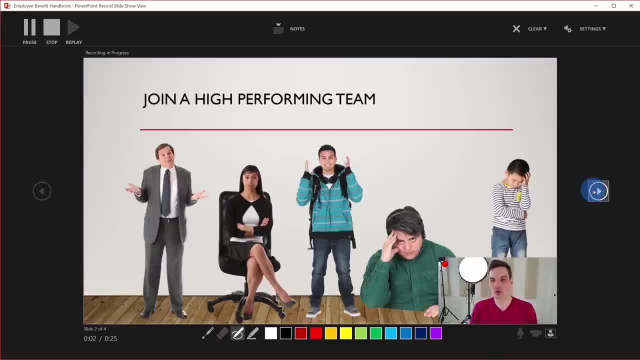 to the next slide. One thing to be cautious of, though, is when you advance to the next slide, that's going to kick off a separate recording. So your audio, your video, basically starts up a new recording on the next slide. So the thing to note is, let's say, you're explaining a point on the first. 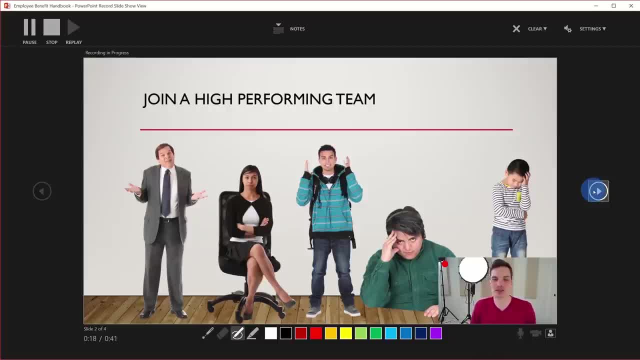 slide and it runs into the next slide. You want to make sure that you pause or you stop before you click on advance and then continue the point on the next slide, Otherwise you'll get this weird cutoff. So I've gone through now, I've annotated my different slides and I'm all done. So I'll go to. 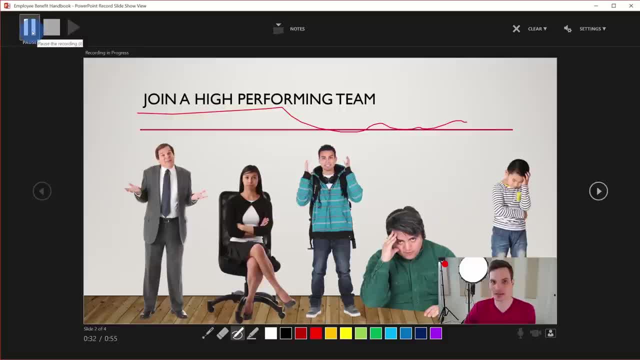 the top left-hand corner and I can now stop it. If I wanted to, I could also pause it, collect my thoughts and then continue, But for now I'll click on stop. My recording is all done now and I can see what it sounds like. I could also go and clear it if, for whatever reason, I was unsatisfied with my. 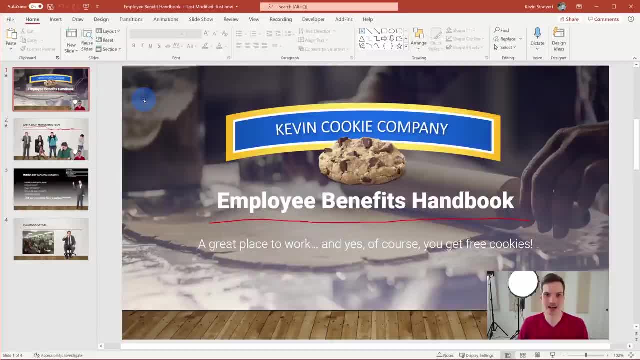 recording, But I think all of this looks good, so I'm going to close this out. This now drops me back into the PowerPoint presentation and you'll notice a few things. My annotations continue to show up on the slide. Here I see my video in the bottom right hand corner. Now I can take my video. 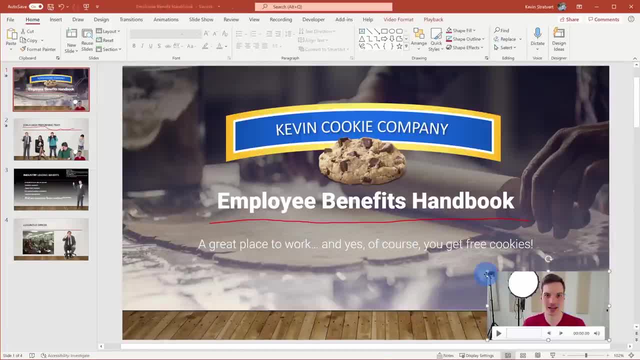 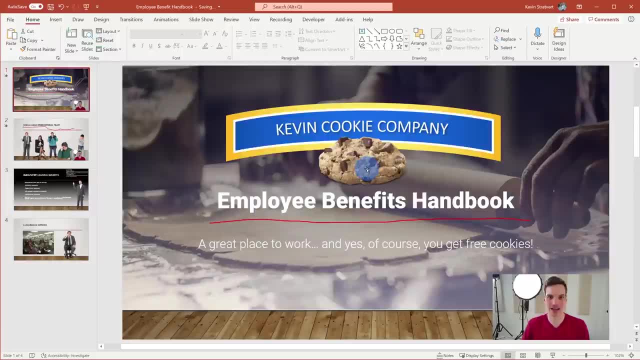 and I can move that around, So I could position it where I want. I could also adjust the size if I want my video to be larger or if I want my video to be smaller. Also, as I was clicking through my slides, I could select track of the amount of time I spent on each slide. So, in a sense, by recording, 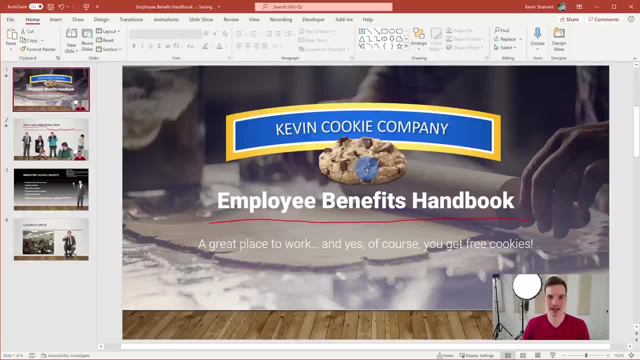 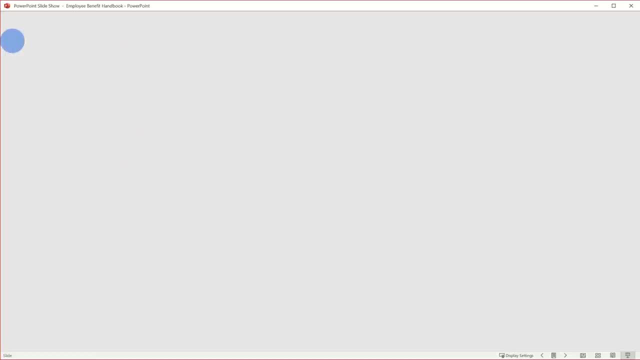 it. you're also setting custom timings for your presentation. If you want to review your recording, you could click up here on slideshow and right here I could start the slideshow from the beginning. Now timer letting me know that the recording is about to start. So right now it's active. 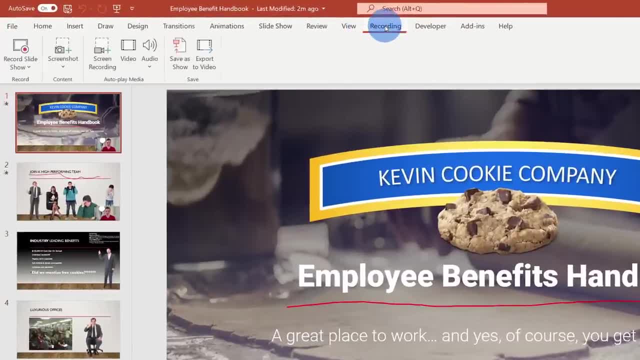 All right. well, that's looking pretty good so far. Let's click back into the recording tab to see what other functionality we have. Now. we took a look at the record slideshow. That's how we added the narration, We added the custom timings, But you also have some other functionality too. 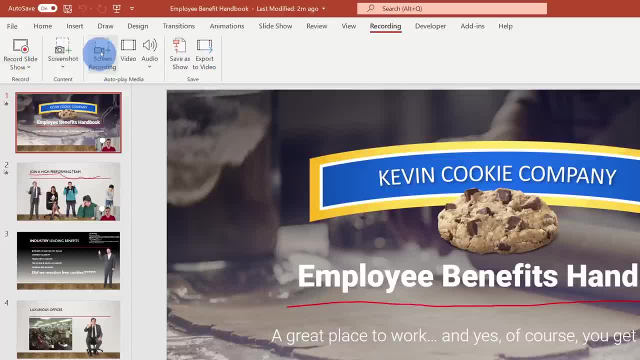 Here, for example, I could insert screenshots. I could also record my screen. So let's say, I want to maybe demonstrate a game, or maybe I want to record some steps that I'm taking in Microsoft Excel. I could do all of that with a screen recording. I could basically record anything. 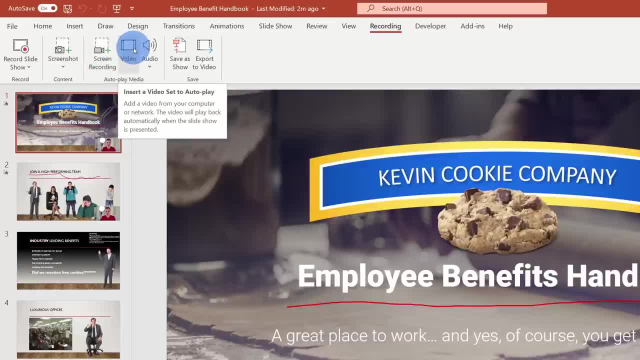 that I can see on my screen. I could also insert a video, and here I can insert audio. You could also use this to insert narrations. Now I do want to show how you can also insert background music as part of your video. So here, when I have audio selected, I'll select audio. 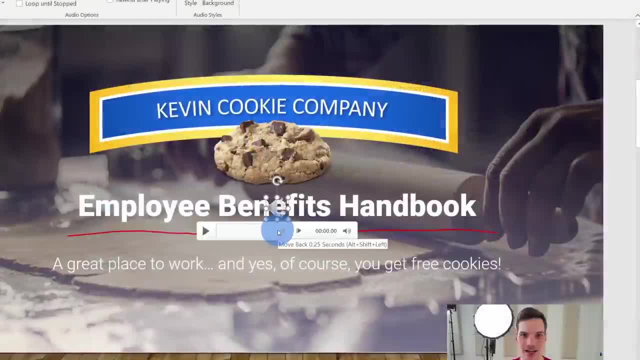 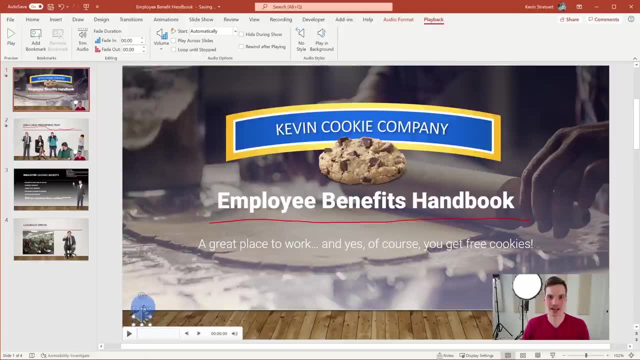 on my PC Here. I'll select this song and then click on insert. Now that I've inserted this song, I can move it to a new position on the slide. I'll place it down there in the bottom left hand corner. When I have this speaker icon selected up here under the playback tab in that ribbon I can select. 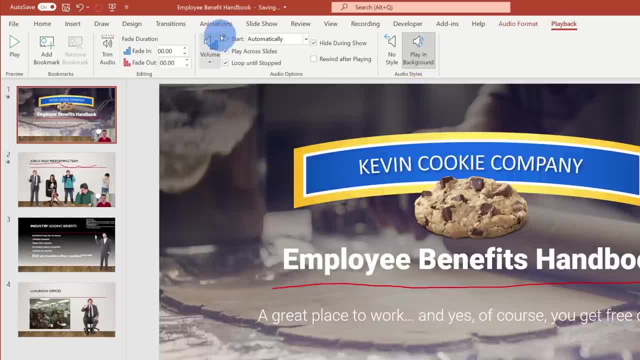 to play this in the background. When I select that, you'll notice that it modified some of these settings in the center. Here I can play it across slides. I could have it loop until stopped and I can have it so it hides that speaker during the 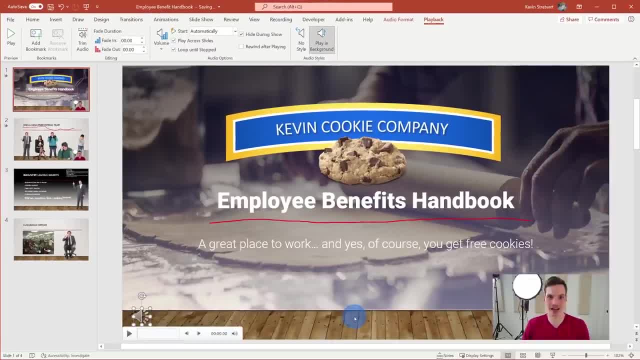 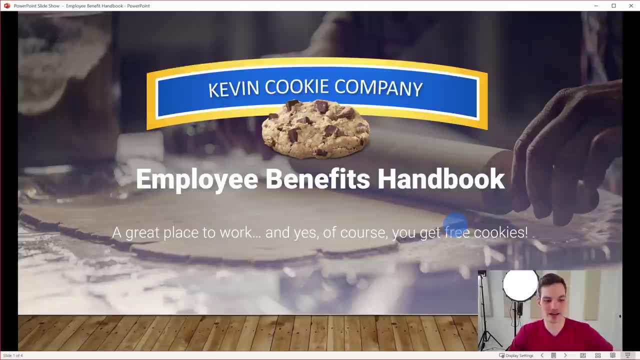 slideshow. So this way now I can have background music play while I'm presenting. Let's test out to see how that works. So here I can select my tools and here I can go in and I can point at things on my slide. All right, well, that's all looking pretty good so far, So I have annotations. 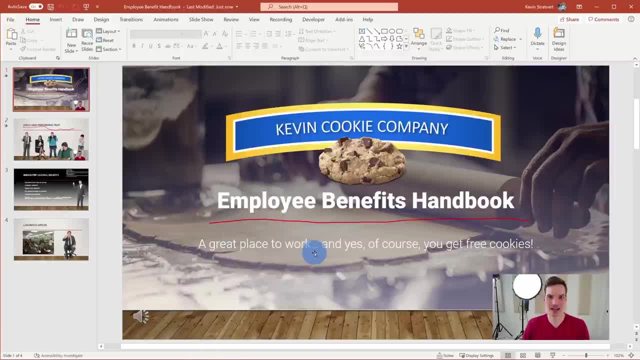 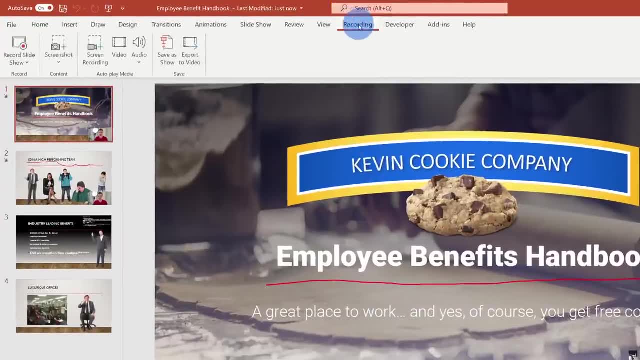 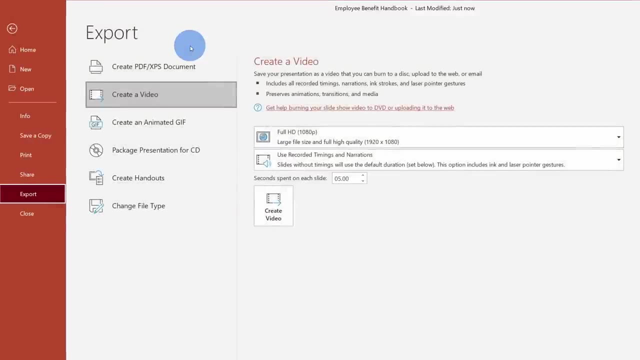 I have narration, I have my video, I even have some background music. Next, I want to show you how you can render this so we can get it into a video format. Up on top once again, let's go over to the recording Tab and all the way over on the right hand side, we can export to video. Let's click on this When. 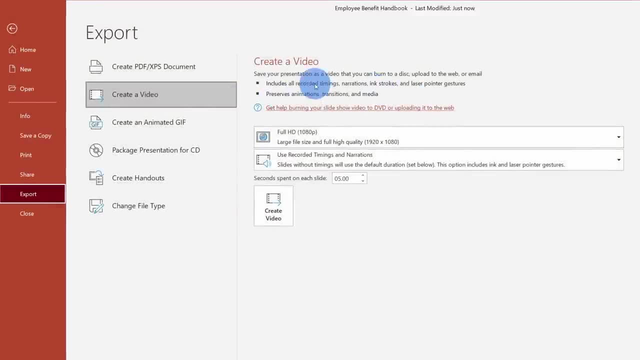 you click on export to video. this brings us to the export screen and we have a few different options here. Right up on top, I can choose the quality that I want to export as, and I can export all the way up to 4k. That's the best quality level, and I always recommend going with the best quality. 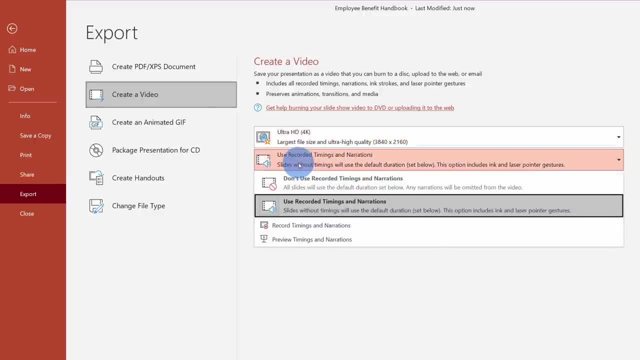 so I'll select this one. Over here you can select to use recorded timings and narrations. So if you go to the slideshow as we advance through the different slides, PowerPoint remembered how much time we spent on each slide, So that's the recorded timing. You could also opt to not. 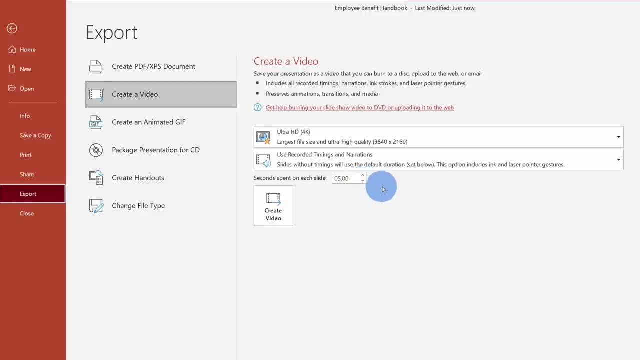 use the recorded timings and you could set your own time spent on each slide. Now I want to take advantage of the recording timings, so I'll leave that selected. Once you make all of your different selections, click on create video. This opens up a prompt where you can choose where you want to. 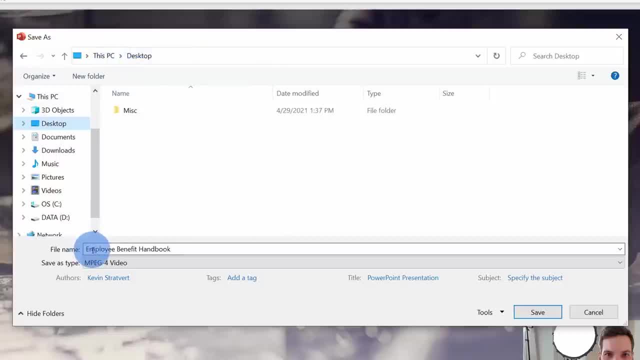 save your video. I'm going to place mine on the desktop and I've titled it: employee benefit handouts. Down below you can choose the save as type. You can save as either an mp4 or a Windows media video For YouTube. I would recommend uploading an mp4, so select that and once you're ready to go, let's. 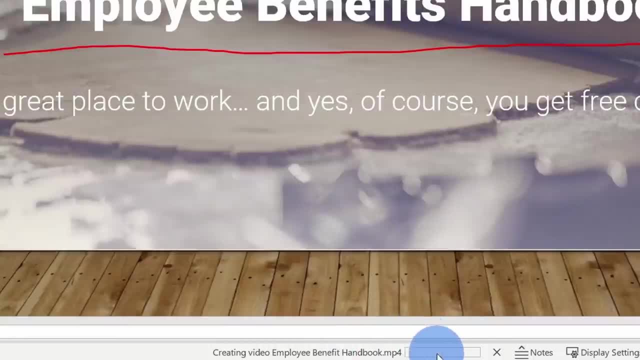 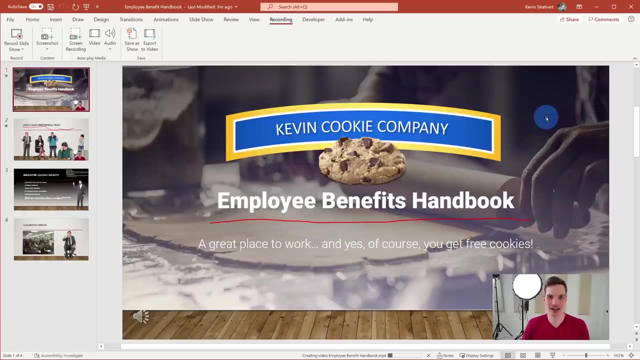 click on save Down below, you can see that the video is now rendering. so since we chose 4k, it's going to take a little bit longer, so you'll have to wait a little bit before your video is ready. While the video is rendering, I want to show you how you can create a custom thumbnail. You can. 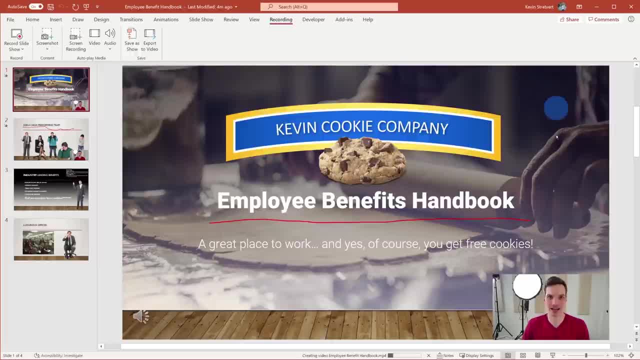 create your thumbnail directly in PowerPoint And I want to use this slide as my thumbnail. but you could also create a separate slide and you could design that slide to be your thumbnail. The really nice thing is the YouTube thumbnail dimensions match the default slide dimensions, so it makes it really easy for you. So here I have. 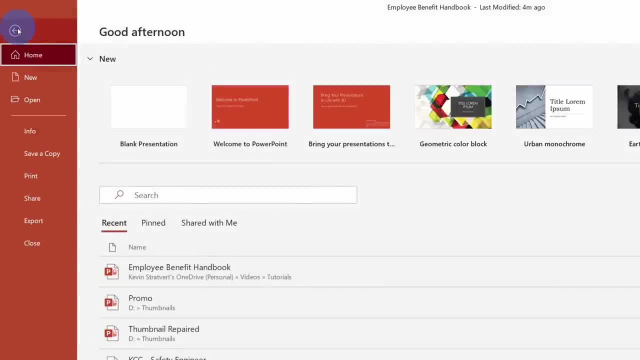 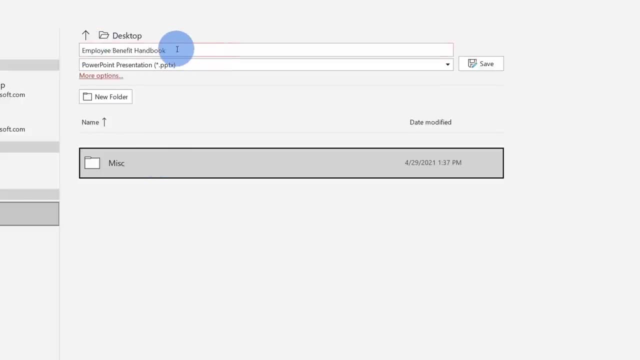 my slide ready to go, I'll go up to the top left hand corner, click on file and then click on save a copy. This opens up the save a copy prompt and here once again I could type in a name for my thumbnail. So by default it's currently set to a PowerPoint presentation, but for a thumbnail I need 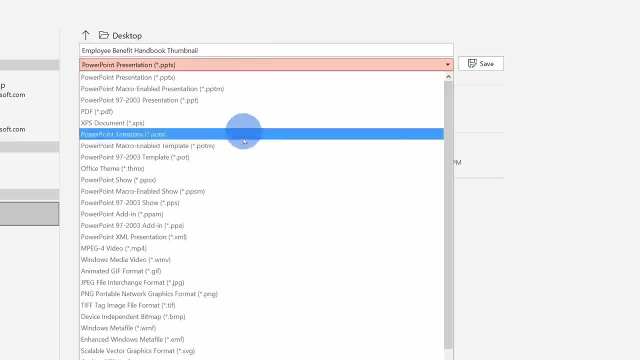 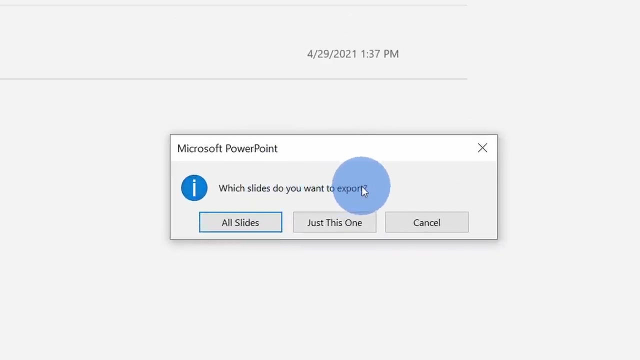 to get it into an image format. When I click on this drop down list, I can save it as a gif, a jpeg or a png. These are three different formats that YouTube accepts. I'll select png, and once you're all done with that, let's click on save. Next, I get a prompt asking me which slides I want to export. 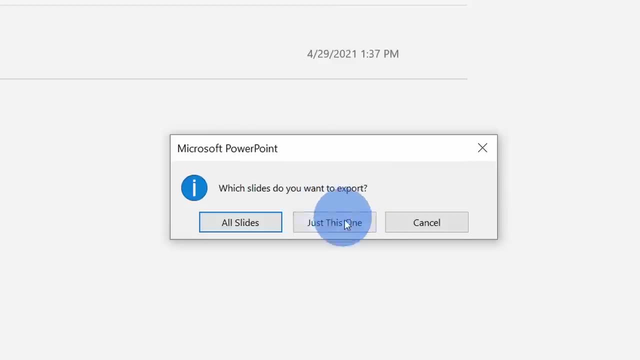 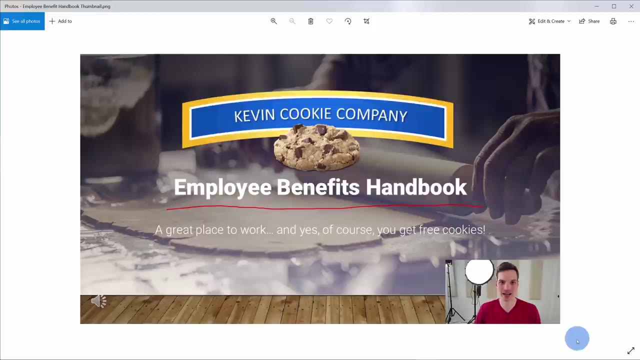 and I just want this one slide to be my thumbnail, so I'll select just this one. I've now saved my thumbnail and that's also ready to go. I just opened up the new png that I created and this looks great. That's my thumbnail. I can use this alongside my video when I upload it to YouTube. 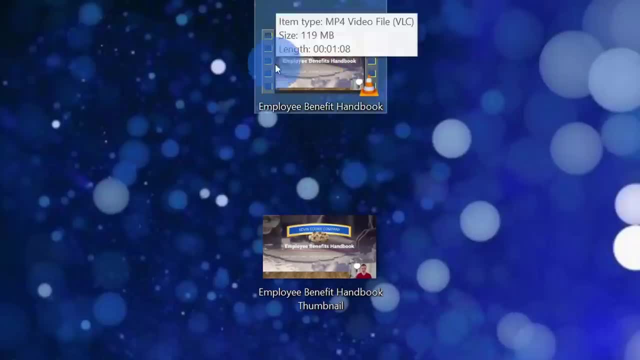 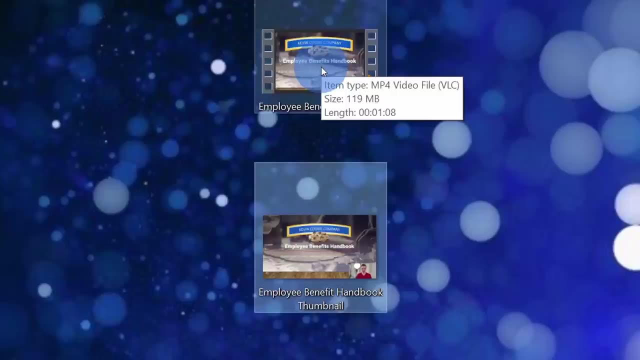 The video has now finished rendering and I now have an mp4 file with my PowerPoint presentation and I also have my thumbnail image. I'll click into the video, just to make sure things look good Now. timer letting me know that the recording is about to start. So right now it's active. 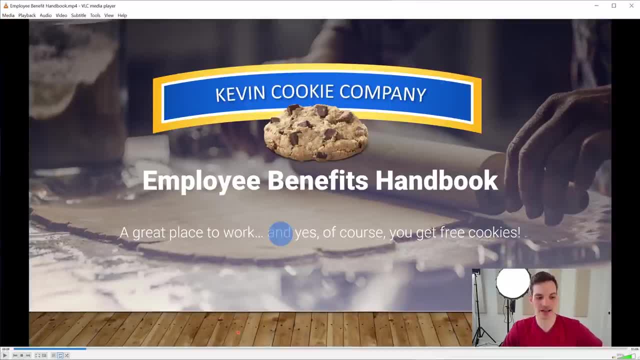 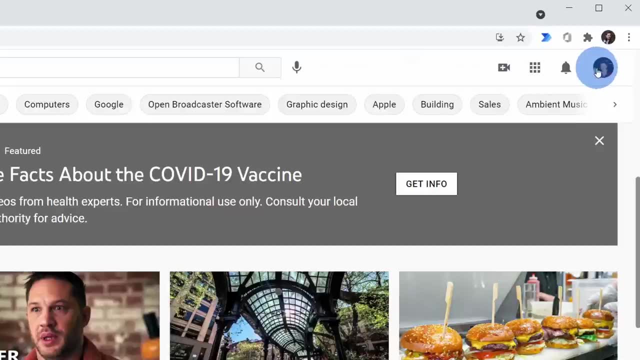 So here I can select my All right. well, I think that looks pretty good. so it's time to upload this to YouTube. To upload to YouTube: head to youtubecom and in the top right hand corner, when you're signed in with your Google account, click on the create icon. This will drop down a menu. then click on upload. 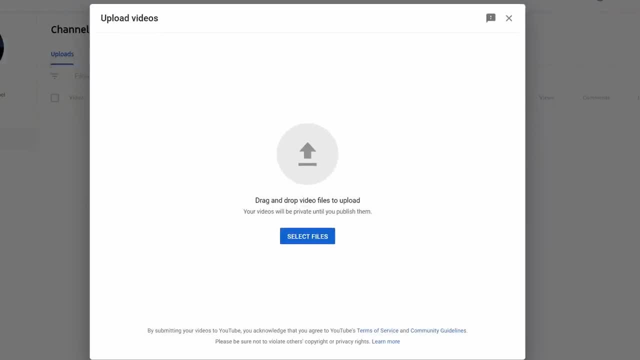 a video. This opens up a prompt where I can drag and drop a video file in, or I could click here to select my file. I'll simply drag and drop my mp4 file over that I created in PowerPoint and I'll drop that over here. so now my video is uploading into YouTube Here. now I can type. 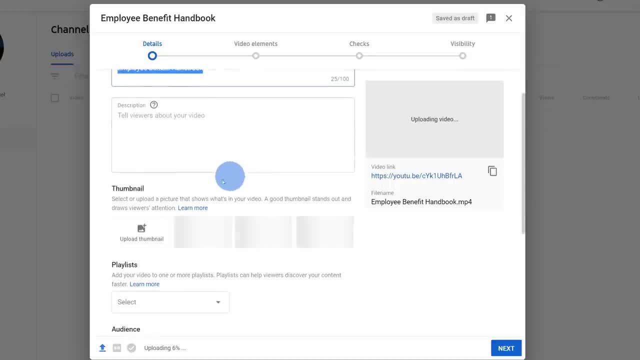 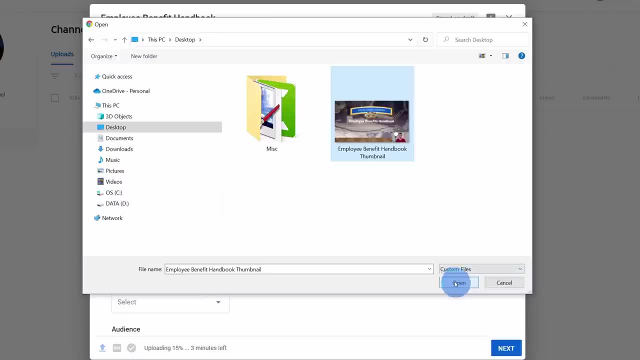 in details of this video. I could type in a title. I could type in a description. Here I'll click on upload thumbnail and I'll select the thumbnail that I saved in PowerPoint. Here's my thumbnail. I'll select this one and then click on open. 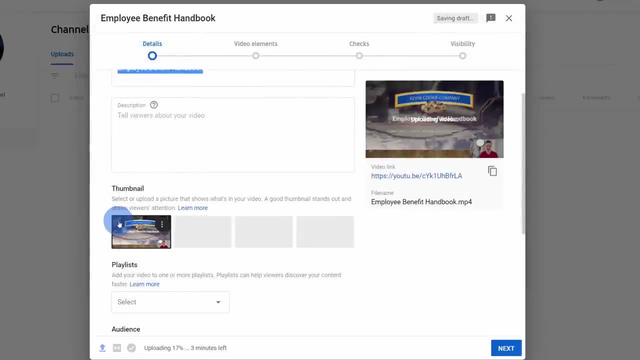 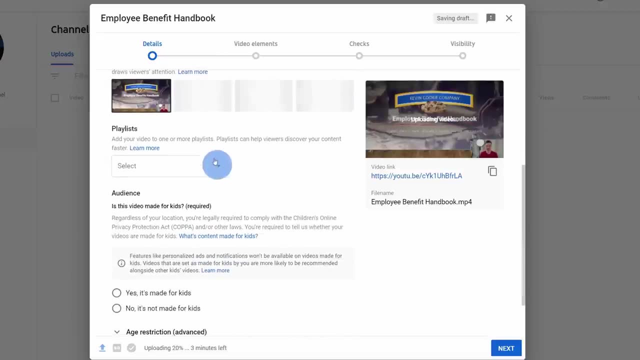 So there you see. my thumbnail now will be associated with this video. Alternatively, if I don't want to create my own thumbnail, I could also choose a still from within the video itself. Here I could go through, I could choose a playlist, I could decide who the audience is. 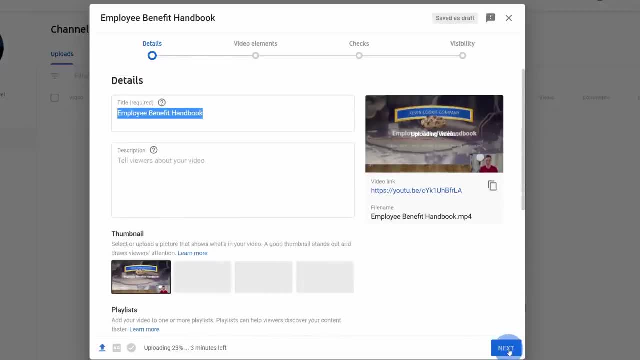 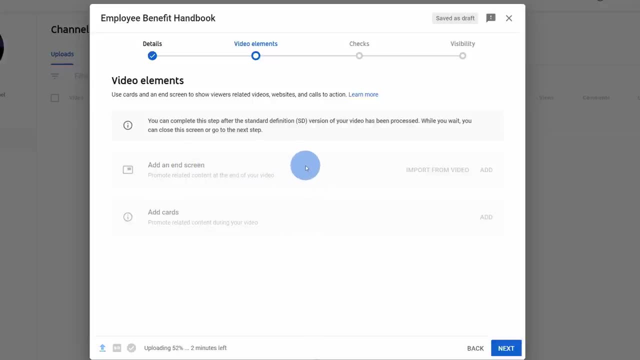 I could add tags. but for now I think all of that's fine, so I'll click on next. On the next screen I could choose to add an end screen. I could add cards. You could even create an end screen in PowerPoint Here. I'll click on next and I'll run through all the different checks. This: 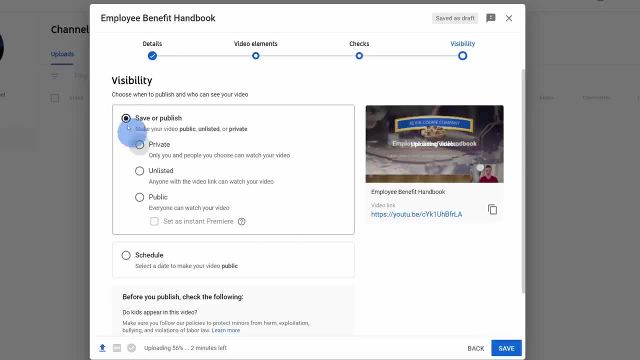 video is pretty safe, so no concerns here. I'll click on next and for the visibility, I could decide when I want it to publish. I could schedule it or I could decide that it goes live as soon as it finishes uploading Here. I'll set it as unlisted for now and then I'll click on save And right now. 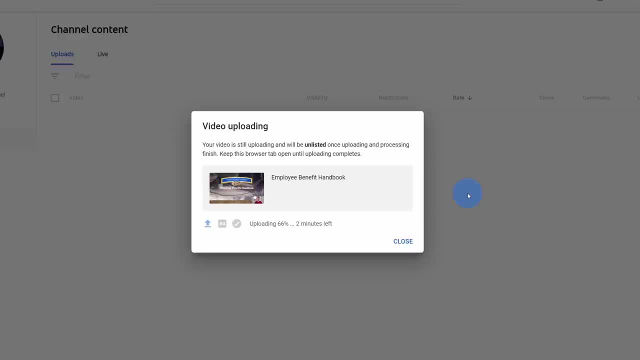 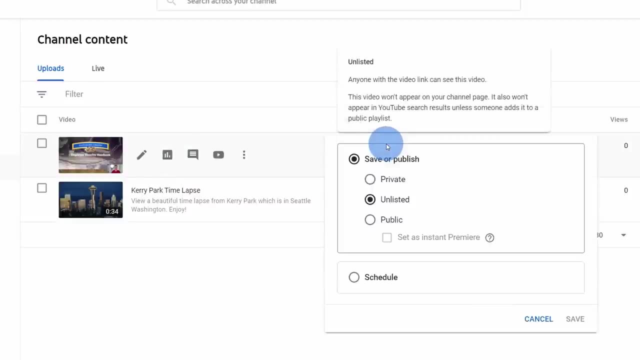 my video is still uploading, so I'll just hang out a little bit until that finishes And it's all done uploading now and it's currently processing the HD version Over here under visibility. I could click on this drop down and I could set it to public Here. I'll click on publish Also when. 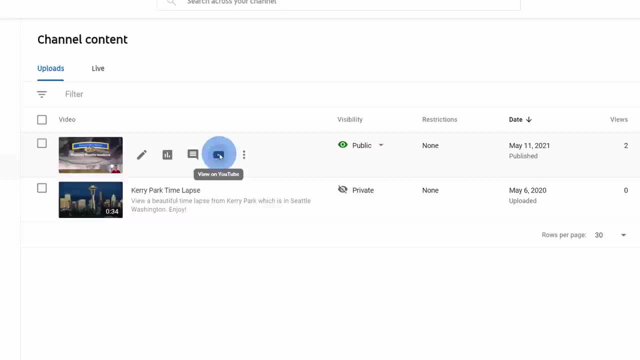 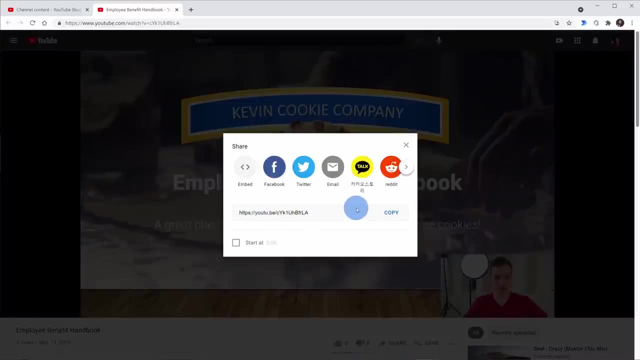 I hover over here. here I can click to view my video on YouTube, And here now I could see my video on YouTube To share with others. I could come down below and I could click on share, and now I could share out my link. All right, well, that's how you can use PowerPoint to create a. 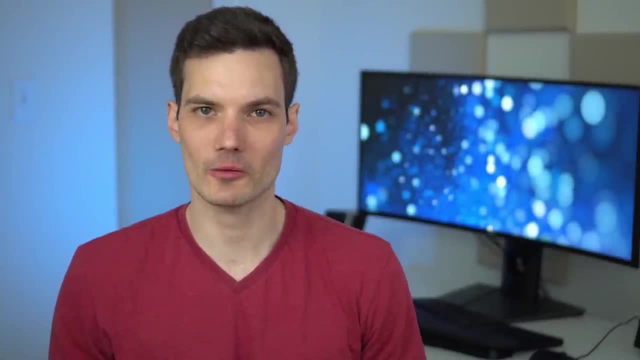 video. Let me know down below in the comments: are you going to use PowerPoint to create your next video? If you enjoyed this, please consider subscribing. All right, well, that's all I have for you today. I hope you enjoyed and, as always, I hope to see you next time. Bye.